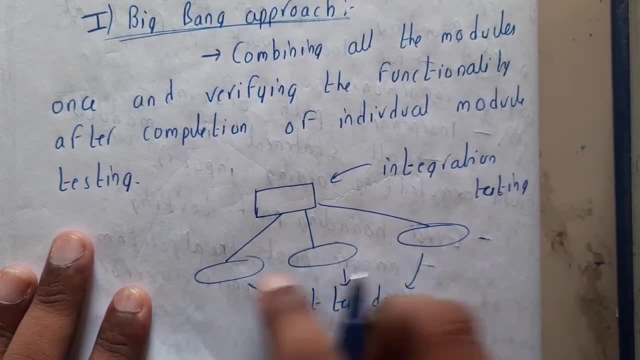 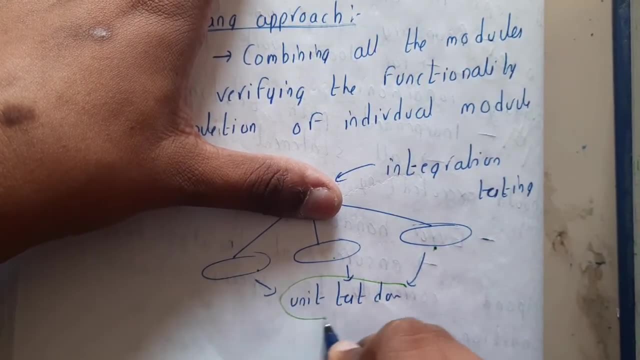 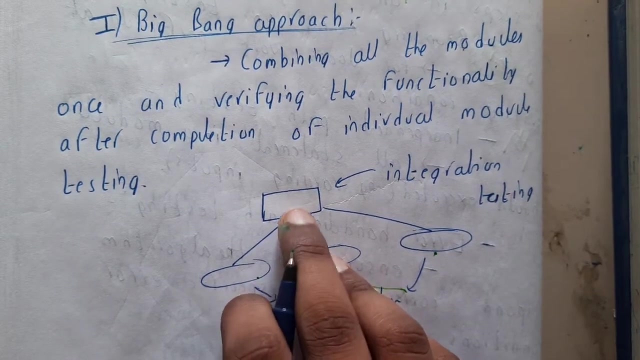 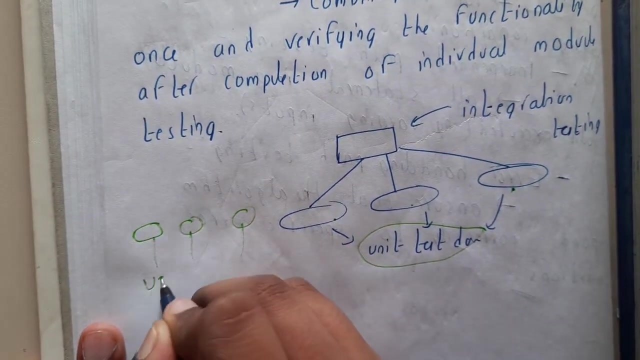 Okay, So you are having three sub modules. So these three are the modules and this is the main module. Okay, So I presume in this way, three individual modules are there, So you will be initially doing the unit testing on individual ones. So once, in individual ones, unit testing is done, you'll be moving, combining them all into one unit and you'll be doing the integration testing. Okay, If you want me to draw a drawing here, guys, So assume these are the three modules. So initially you'll be doing solely unit testing. Okay, So once unit testing is done, you'll be combining them all and a big model will be made. So this is the model. 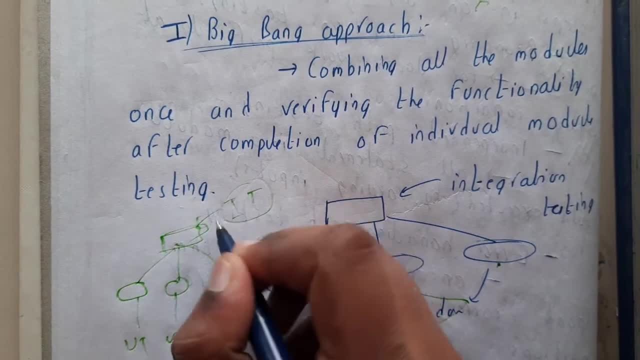 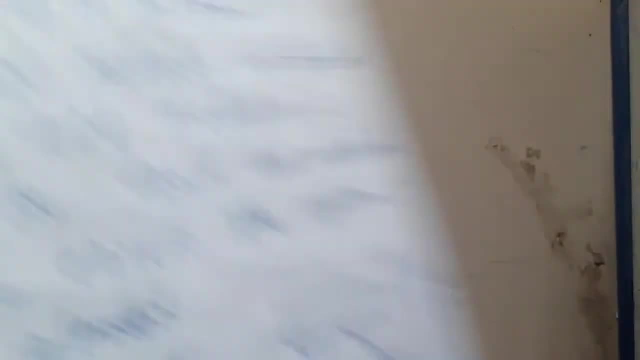 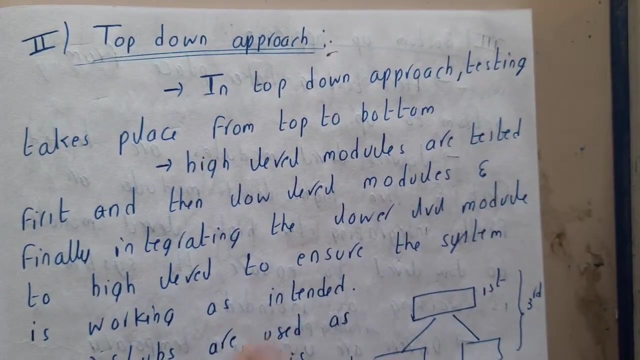 created and for this you will be move, you will be doing the integration testing. fine, okay, so in this way it will be happening, guys, okay, okay, just give me a second. okay. so similarly, top down, top down approach. so basically, top down approach from top you are going to down. so please remember in that, 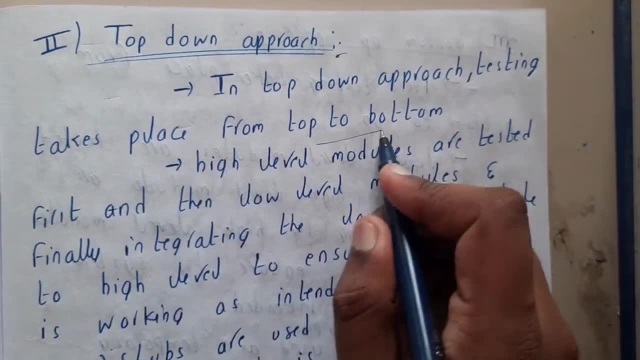 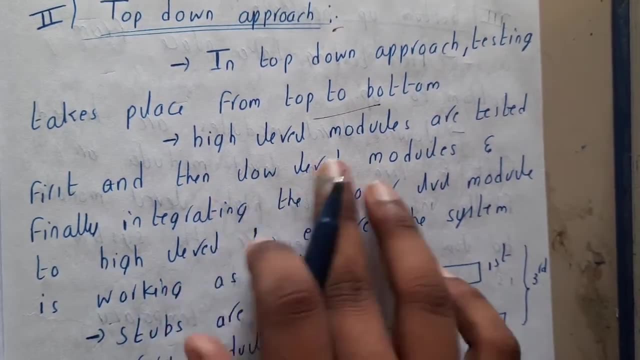 way. okay. so in top down approach, testing takes place from top to bottom. okay, high level modules are tested first and then low level modules are tested. okay, so it's clear. right, it's up to the point. and finally, integration: integrating the lower level modules to the higher level is ensuring. 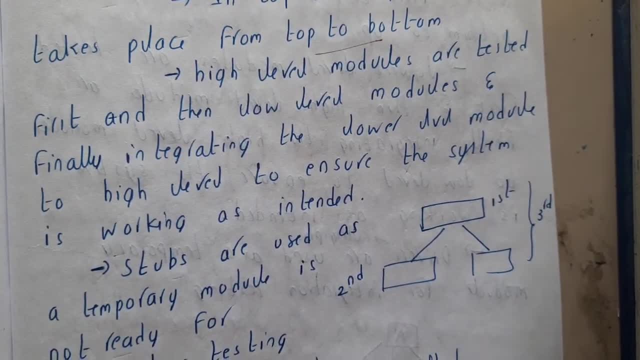 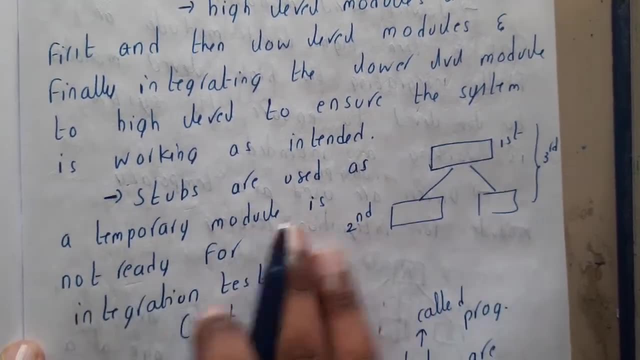 that it is working fine and without any technical issues. okay, so here we will be using a concept called stubs. guys, we'll be discussing about that, don't worry. stubs are used as temporary modules in the modules when module is not ready for integration testing. so you can assume that as 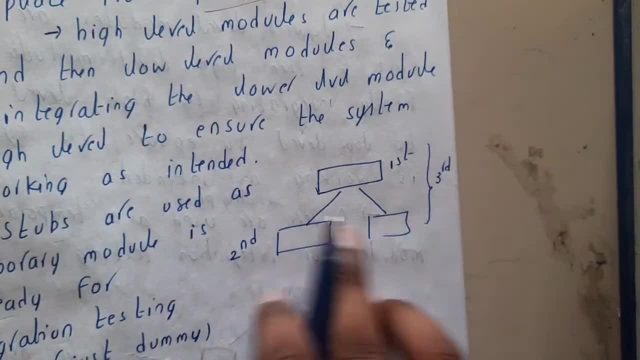 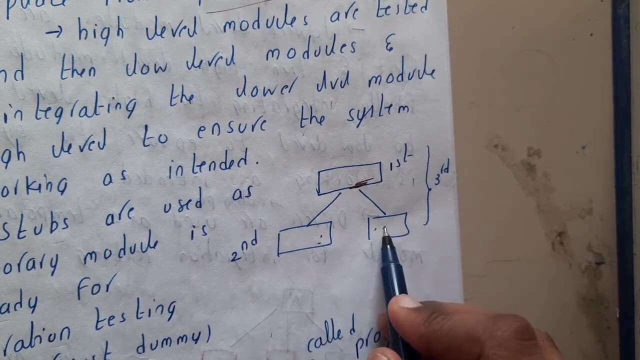 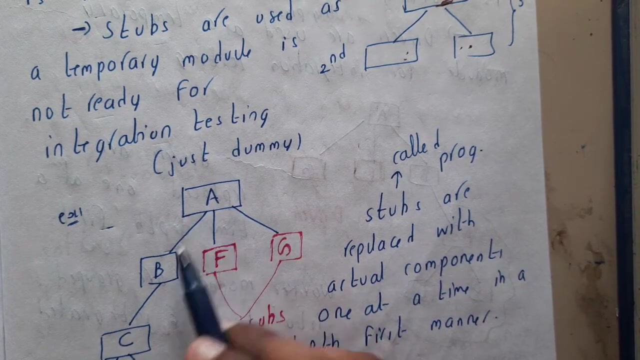 just a dummy, guys, okay. so if you just draw a graph like this or a tree like this, so you'll be having on top, you'll be having the main module and these two are the child modules for the inside. that okay. okay. so assume that you are having a big module, a guys, and for a we are having three small modules, or you come. 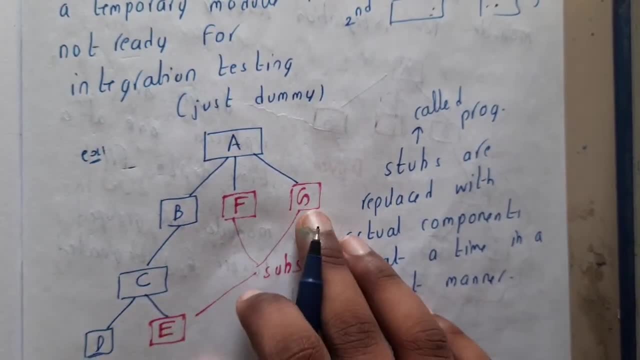 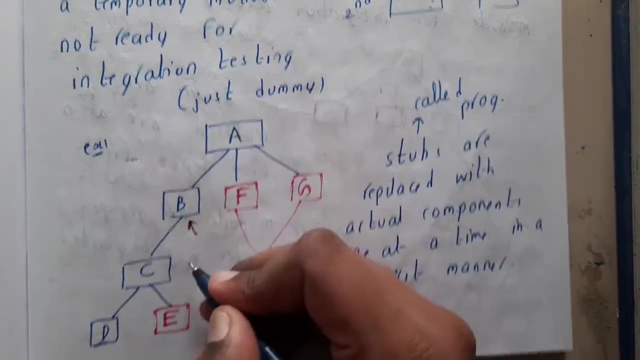 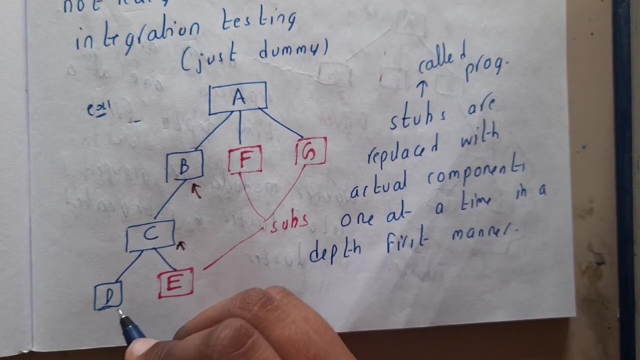 from bottom also, anything will work. so a, f, g, only b's unit testing is done, guys, and f and g unit testing has not yet completed. similarly, here we are having c, from b we have gone to c and from c we are having two modules. again here d's unit testing is done, whereas e's unit testing has not. 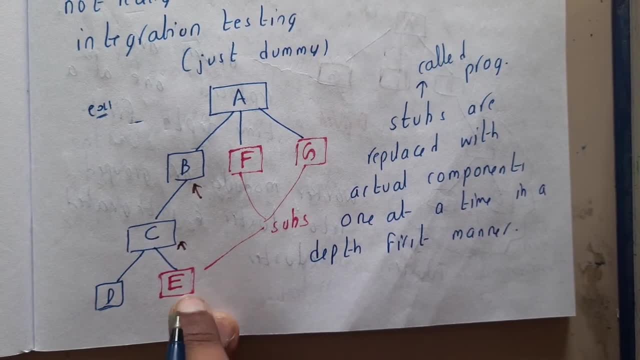 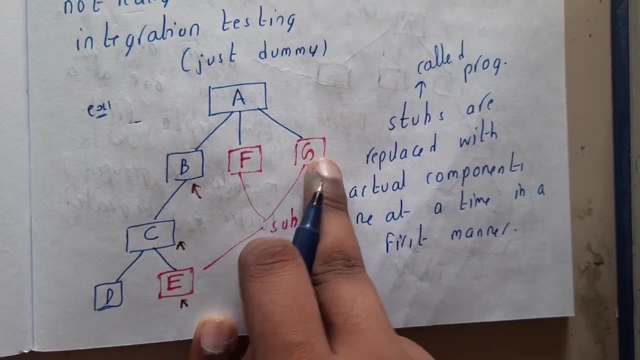 yet done, so for unit testing not done. modules: you will be maintaining some dummy modules until the unit testing is done. you'll be maintaining them only. so the pink color i wrote i drawn here right. so these are dummy modules. so using this dummy module, we combined them and we made into c. 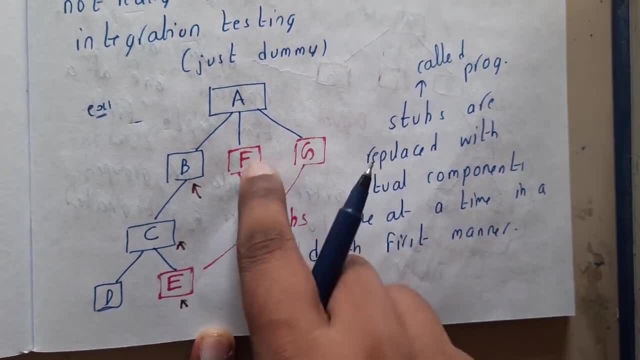 using c. we made b using b, f and g. these two are dummy modules. we made a and we are testing a now. so whenever these are done, this unit testing is done. so we are having two modules. again here, d's unit testing is done, whereas e's unit testing has. 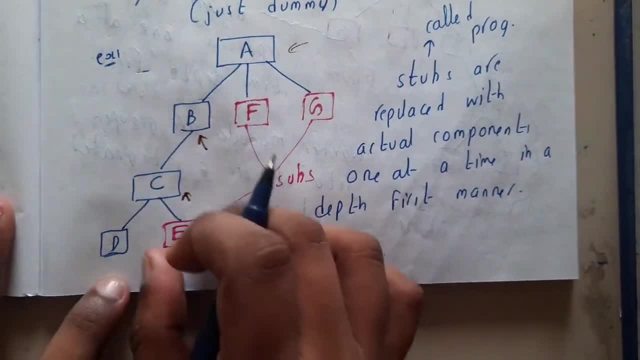 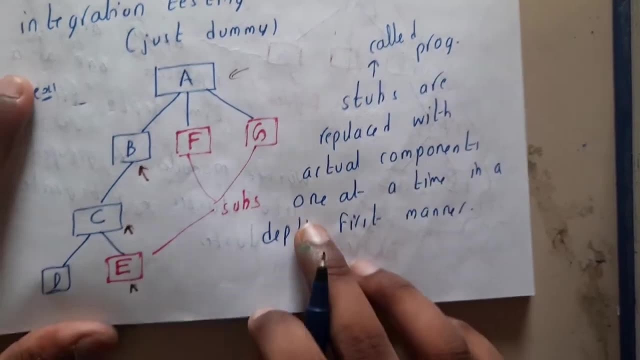 done so, original e- then you will be inserting that and you'll be again, you'll be performing the operation. so stubs- stubs are called stubs- are replaced with the actual component, once, one at a time in a, in a depth first search order. so again, remember it will be coming from the depth first. 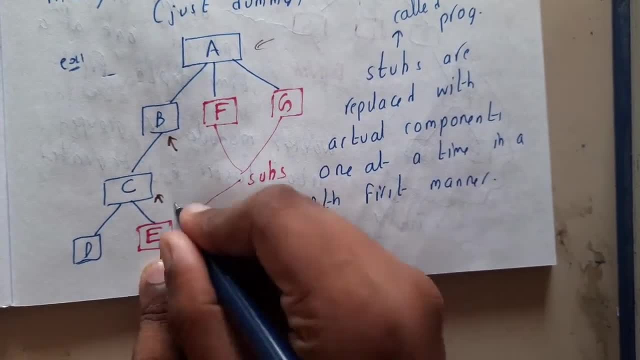 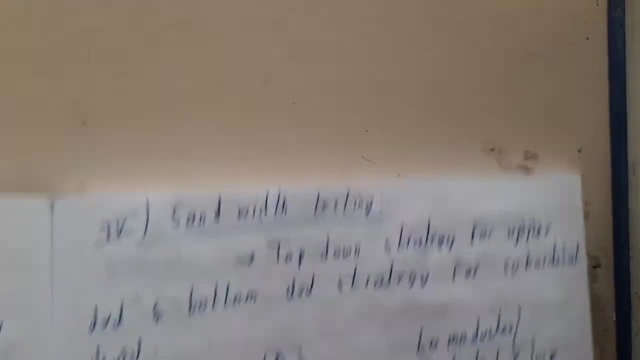 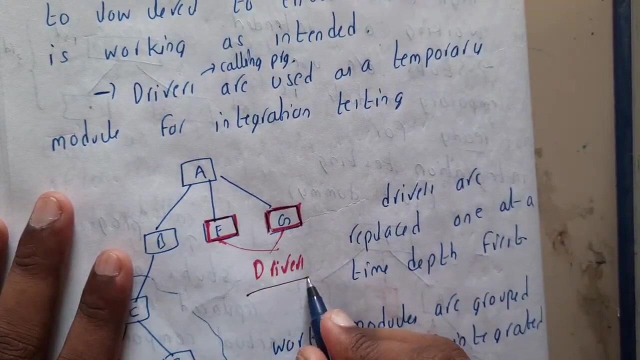 search. so on this side, this is the depth. so first, this will be done, okay. second, this will be replaced. and third, this will be replaced once their unit testing is done. please remember that also, okay. so the opposite of this is nothing but bottom up approach. so in this also we are having, so that duplicates here we will be calling them as drivers guys, okay. 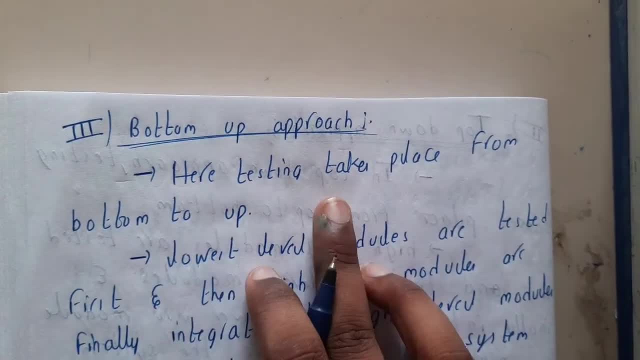 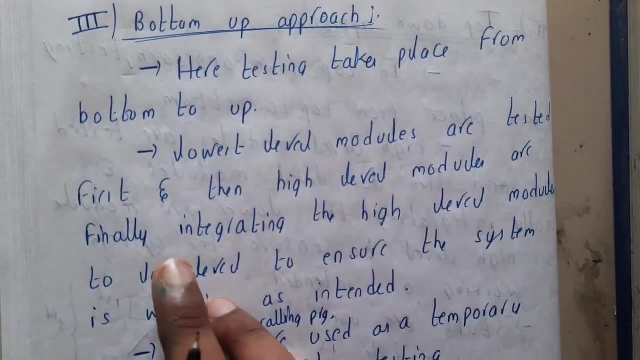 so let us go through the theory, then we'll be going through example. okay, here testing takes place from bottom to up approach, so the lowest level modules are tested first and then higher level modules are. finally integrated- the highest level modules to the lowest level to ensure the 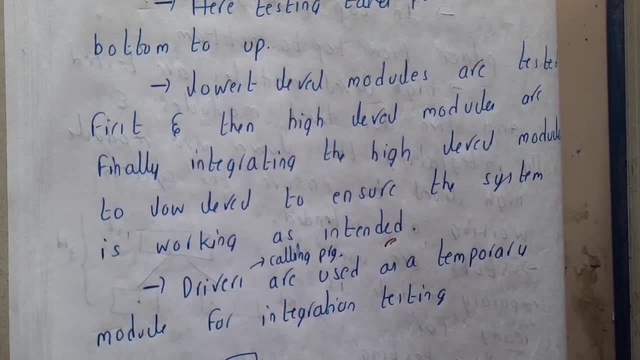 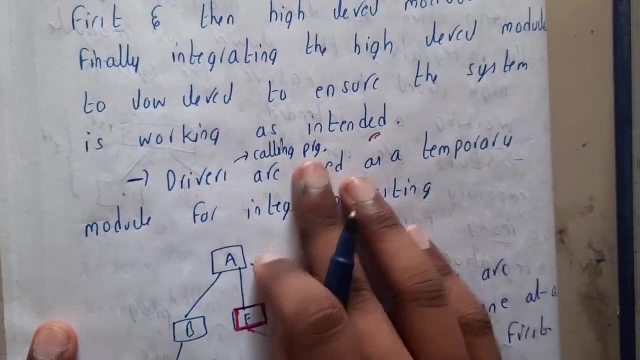 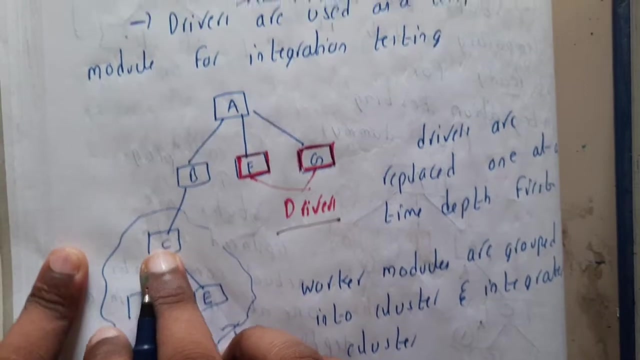 system is working as an intended, as intended. so, basically, here you will be, just you will be reversing the approach, guys, from bottom to top you will be doing here. so drivers- here we will be using drivers called are used as the temporary modules to integrate the testing. okay, so i told you from bottom right. so here we are having all modules, so you done. 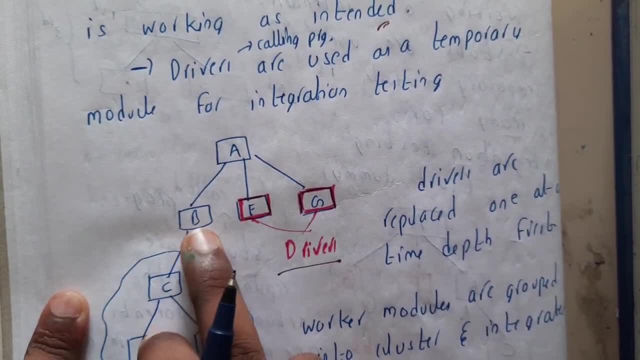 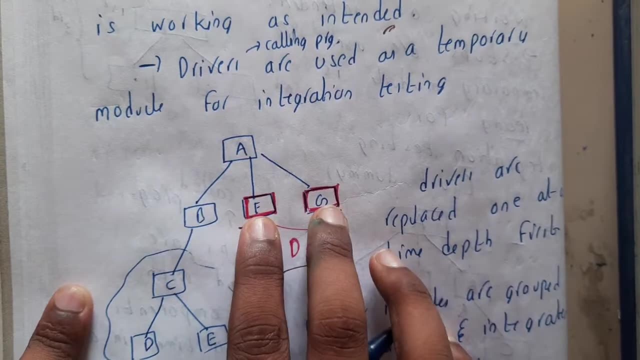 you done it there safely, so you came to b from b, f and g. so you are not having f and g are not yet completed their unit testing. so now you will be creating two dummies and you'll be placing them and you'll be completing your integration testing. whenever these two are ready you'll be replacing. 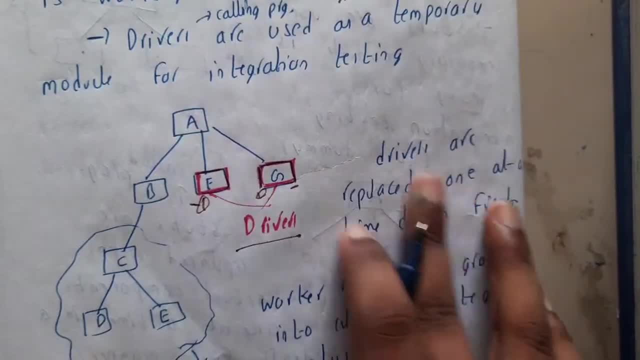 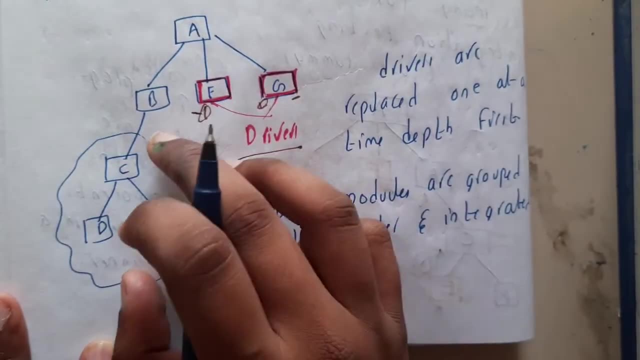 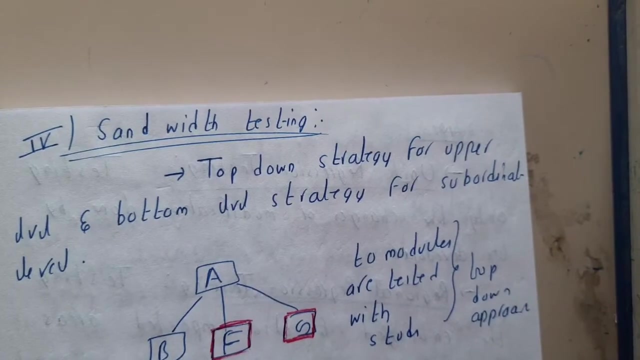 them in the depth. first, search order, first f and second g, so drivers are replaced one at a time. order: worker modules. so these modules, like 100 working modules, those segments, like you'll be breaking them into some parts and each part is called as cluster. okay, okay. so the last type of